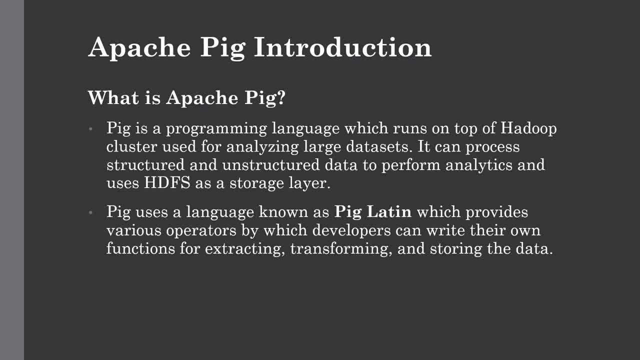 is a scripting language used for processing either structured, semi-structured or unstructured data as well, And it can use Hadoop for resource allocation as well as the storage layer. So it uses yarn for resource allocation and HDFS for storing the data. So, as I have said, it uses the pig Latin, which provides various operators, So it is just like a SQL language. So if you're familiar with SQL, this is pretty much very easy to understand for you. So to 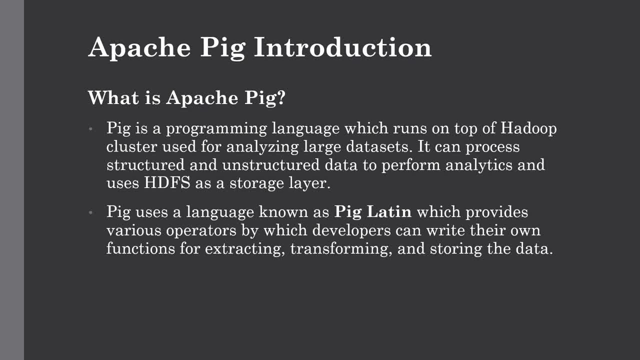 analyze, analyze data in apache pig. so we need to write script using pig latin language and you can execute it on our hadoop cluster as well. so on the higher level it will just convert that pig script into the map reduce job, in which our program will be converted into mapper. 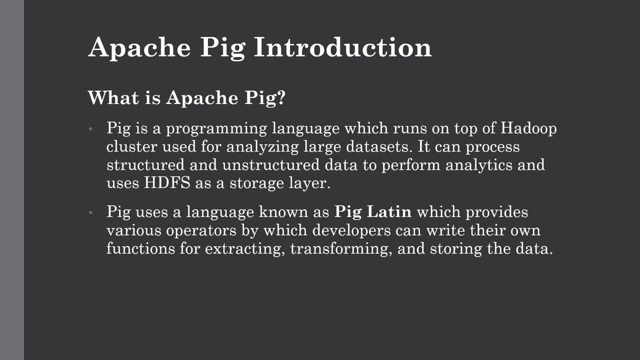 and reducer programs and it will be executed parallely across our cluster. so, as you already familiar with the map reduce, we don't need to discuss that in detail. but apache pig is just like hayu, but hayu is more or like used for processing structured data, which is in 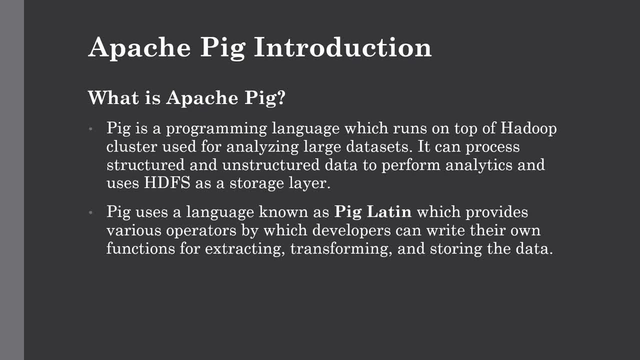 form of tables, just like rdbms, and it is also similar to a database system. but coming to apache pig, it is more versatile tool and it can handle structured as well as semi-structured data as well. but wait a minute, we have other processing languages, so why we need it actually? 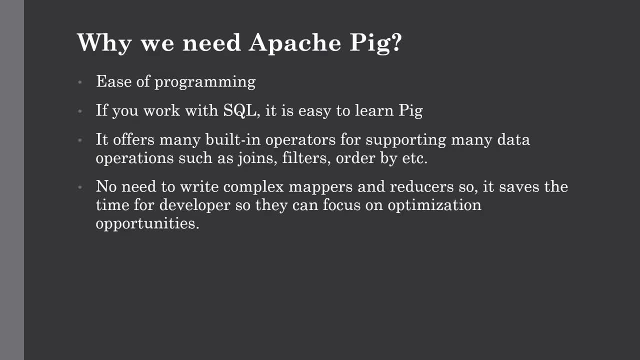 that we will discuss now. so basically, the major selling point for apache pig is the fact that apache pig is not just a database, but it is also a database system. so what does it mean really? so the developers who are not good in java will normally struggle working map, reduce jobs for processing the data on hadoop because, as you already know, 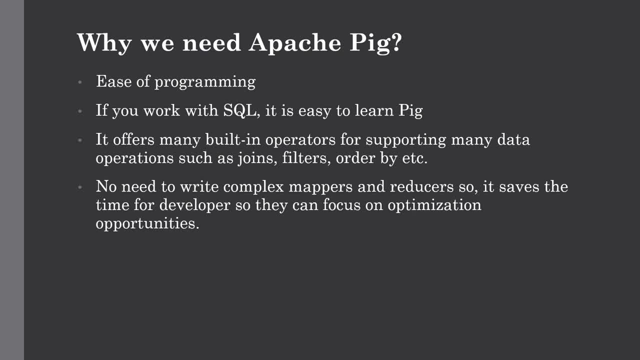 map reduce jobs are majorly written in java and it could be very complex, so a certain small operations can become several lines of course, which is not that efficient for every developer. so if you go for apache pig, that pig, latin language is very simple to understand. the second point is obvious. so if you work with sql, it will be very easy. 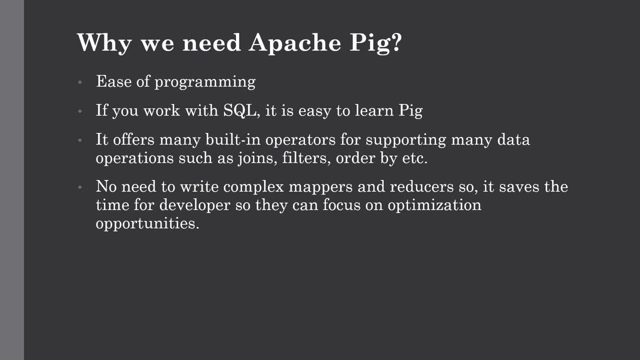 to learn pig, because, after all, pig is also a scripting language and the syntax is pretty much similar to the sql which we have discussed in our hayu tutorial. the next one is it offers built-in operators for supporting many transformations, such as joins, filters, order by, etc. so just 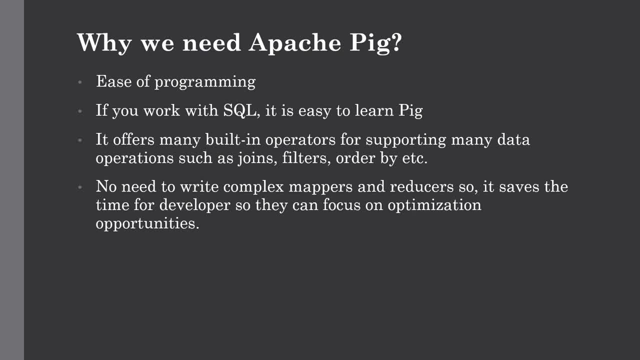 like sql, we can either join two or more data sets as well as a project, or we can either supply filters to it and use order by for sorting out the data. so it comes in handy if you're dealing with structured as well as semi-structured data. and the last and most, 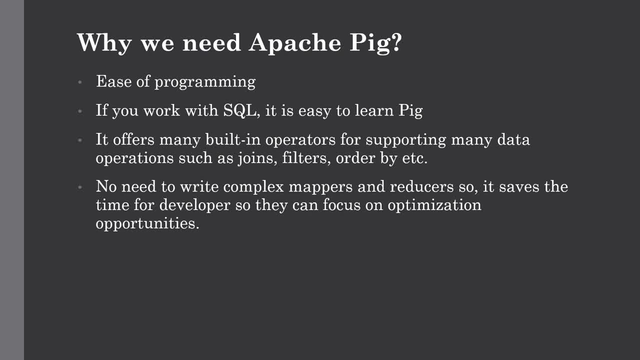 important. you don't have to write complex mappers and reduce a function, so it will save you a lot of time. so, as a developer, you can focus on optimization opportunities, which is way more important if you're dealing with huge number of data sets. so this was all about. 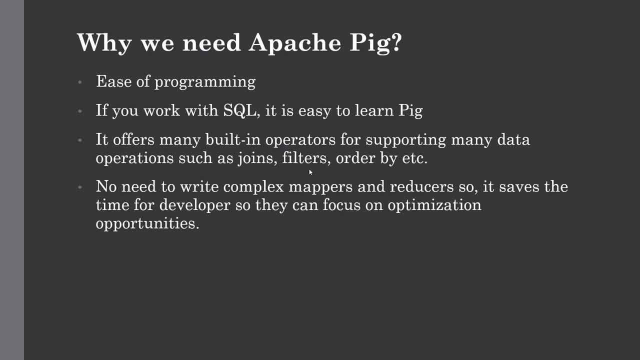 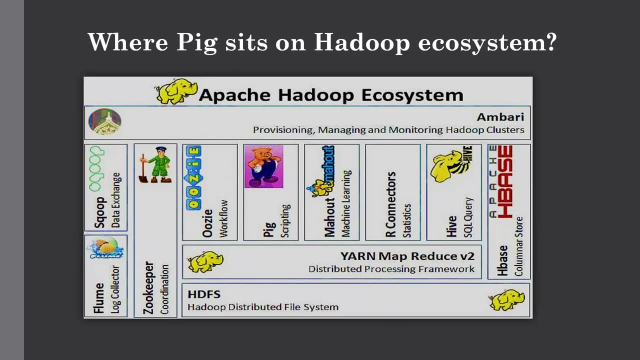 why we need the apache pig. but you may ask, where does it actually sits? on our Hadoop ecosystem, so let's discuss about that. so, as you can see in this representation, apache pig is nothing but a scripting tool which sits on top of MapReduce. so what it will does is if you submit your pig script, 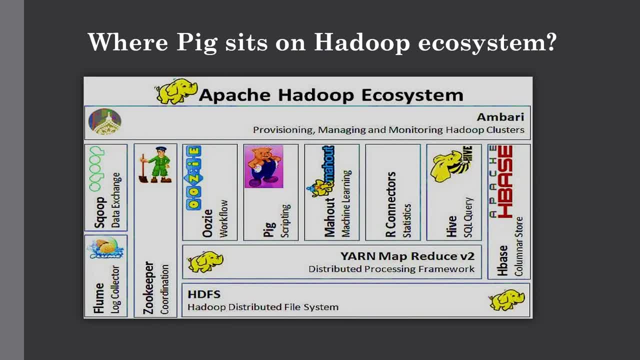 on Hadoop cluster. it will just convert it into the MapReduce job, where the mappers and reducer functions will work to provide the solution and process your data, and it will use yarn as a resource allocator so it will communicate with your name nodes and data nodes simultaneously. 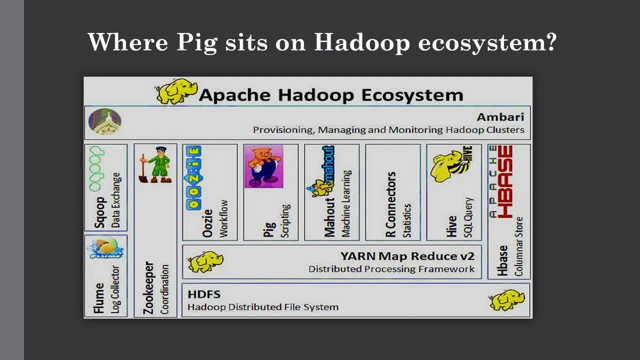 to get the info of where the data resides and how to process it. it plans and submits those parallelly to get the benefit of parallel processing of the distributed computing. so it can also make use of Tez execution engine. so you may remember when we discuss in Hadoop. 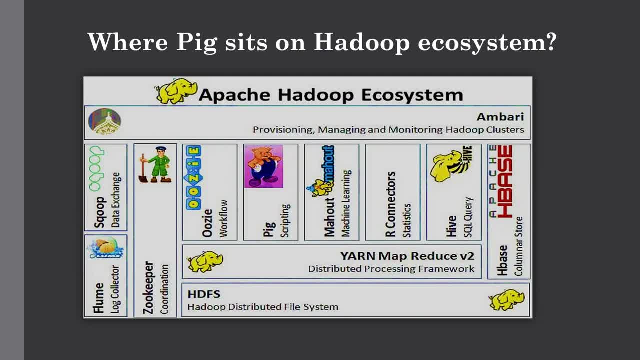 there was one execution engine which can be an option for MapReduce, so Tez engine will take the advantage of the DAG, which is direct acyclic graph. so rather than making it a linear process like mappers and reducers, it will find the most optimal way by finding the correlation between all the tasks which needs to be executed parallelly. 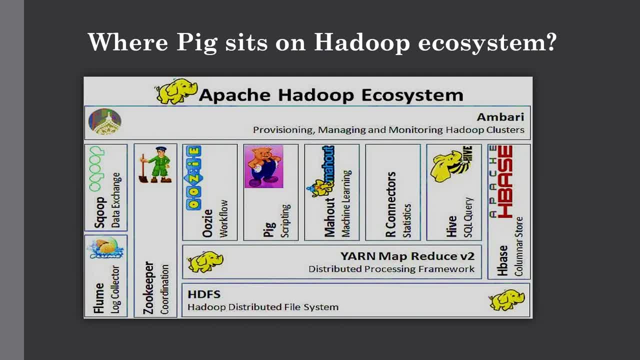 and it can give you up to 10 times faster execution than MapReduce. so what it is actually, that we will see in our upcoming lectures and we will also make a comparison between using MapReduce versus using Tez execution engine for both Hadoop and PIC- and we will see the difference. 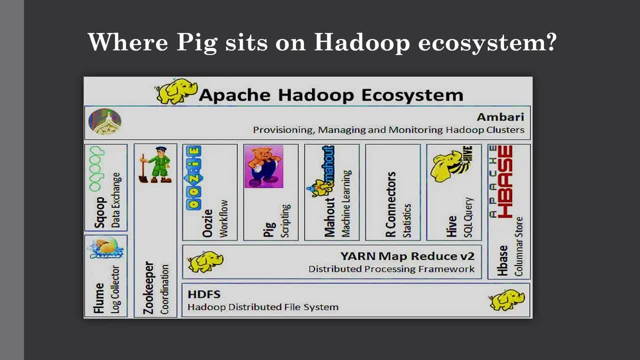 and see the power of Tez, and you may also be aware that this DAG, which is direct acyclic graph, this concept is also used in Apache Spark for getting faster computation of your data. but simply said PIC, nothing but sits on top of MapReduce as well as Tez to process. 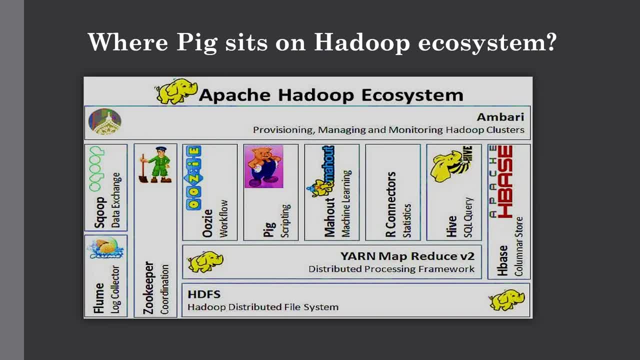 your data so that PIC script will be converted into MapReduce, or either the Tez job, which again computes the data on top of your Hadoop cluster by using the YARN as a resource allocator and the HDFS for storing the data. so this was pretty much all about where this PIC sits. 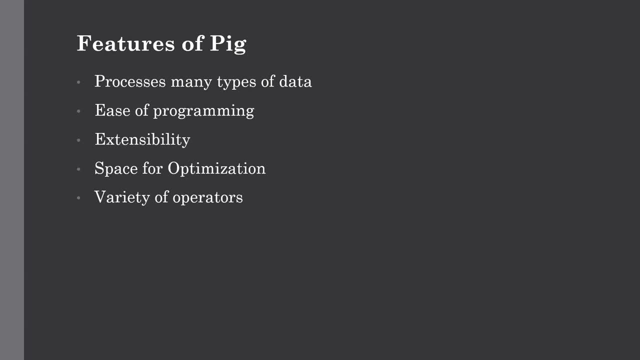 on our Hadoop ecosystem. so at the last, let's discuss about some key features of Apache PIC. so the first one is it processes many types of data. so what do I mean by that is it can handle all kinds of data, such as structured, semi-structured and even the data processing. 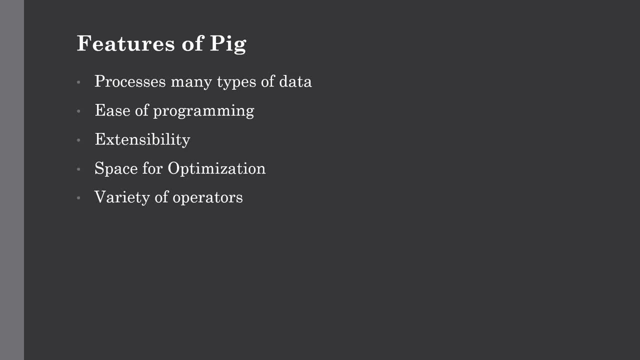 of the data. It can handle all kinds of structured data as well as the unstructured data, which is the key selling point for using the Apache PIC over the Hadoop, because Hadoop can only deal with the structured data which is present in the form of table, like structure similar. 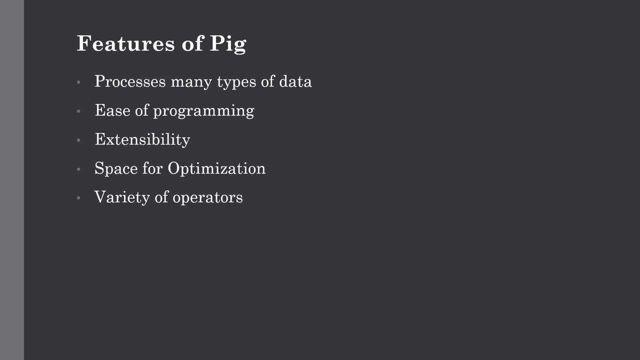 to the RDBMS. the next one is ease of programming, so you don't have to worry about writing long scripts, which is written in Java, which has the mappers and reducer function to it. you can just use the PIC Latin language, which is just like SQL, to process your data and 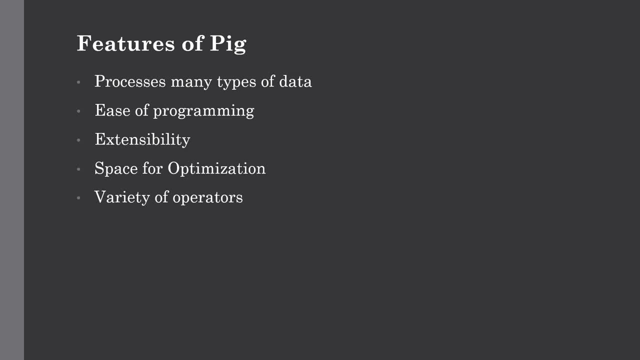 it can, automatically converts it into the MapReduce job and submit it on the Hadoop cluster, so you don't have to worry about writing a big Java code. so if you're a SQL programmer, PIC Latin will be easy for you to understand. you will get more clear idea in our next lecture. 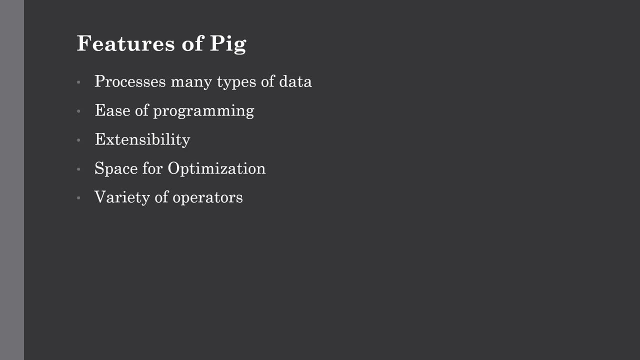 where we will actually submit the PIC script on our Hadoop cluster. the next feature is extensibility, so it is the most interesting feature it has. so it means that we can use our own function For reading, processing and writing the data using the existing operators present in Apache. 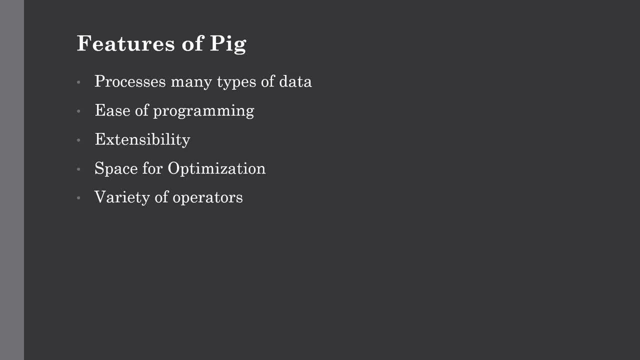 PIC. the next one is it has the space for optimization. the benefit of working with PIC is the task: optimize the executions automatically, so don't have to worry about that, and we can only focus on the semantics of the language. and as you don't need to spend more time developing your